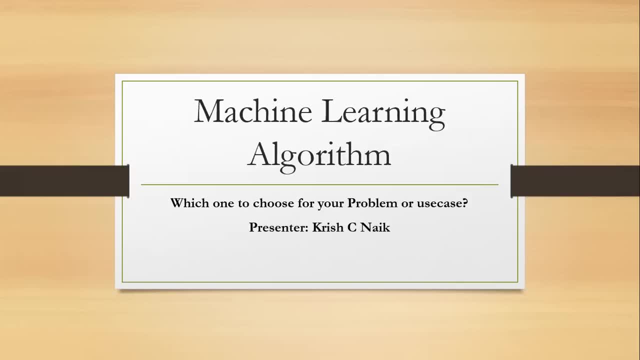 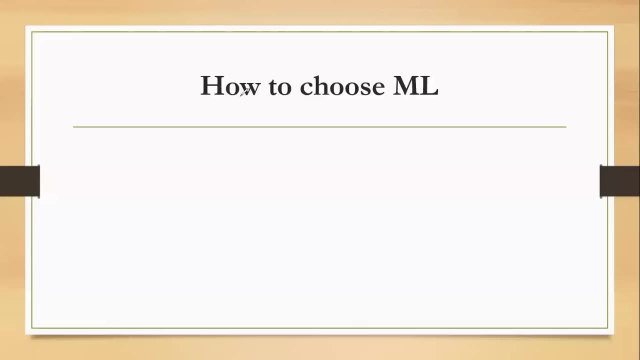 so make sure you watch this particular video till the end. so, to begin with, what we are going to do is that we will just understand some basic concept like: how do you decide to choose? which machine learning algorithm should I basically use? now let me just consider whenever you have a use case- and when I say use case, this is basically for a supervised 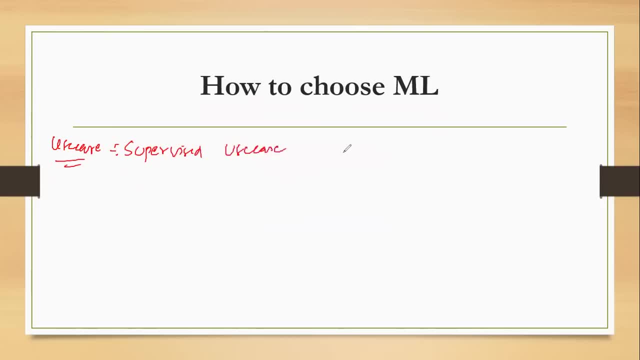 machine learning statement or supervised use cases. that basically means that this is for a supervised machine learning problem statement. that basically means that I will be basically be having a data set, you know, and this data set may be a classification or regression problem. may be a regression or classification problem, right? 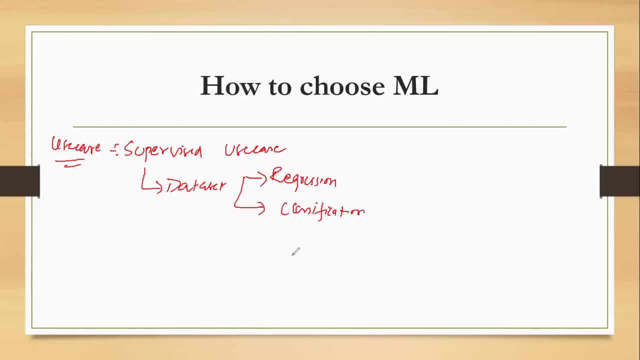 it may be anything of this too. then I'll show you some techniques. you know, some techniques that we should always apply before, as soon as we get a data set, you know. so that will actually help you to select the best machine learning algorithm that will be suited for. 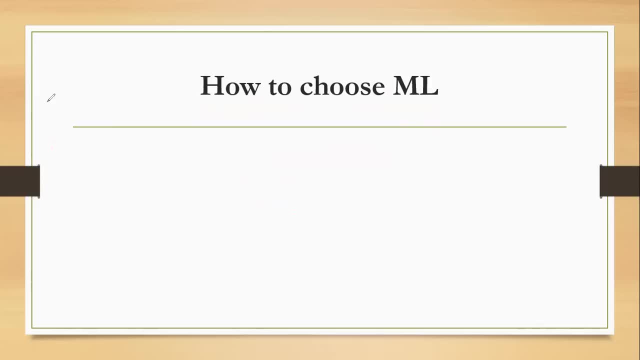 this particular data set. so let us just go ahead and understand it, suppose. let us consider now a classification problem statement. and you know that for a classification problem statement We have various algorithms. first of all we have machine learning, more algorithms like logistic regression. it is a classification problem statement. the second thing can be: 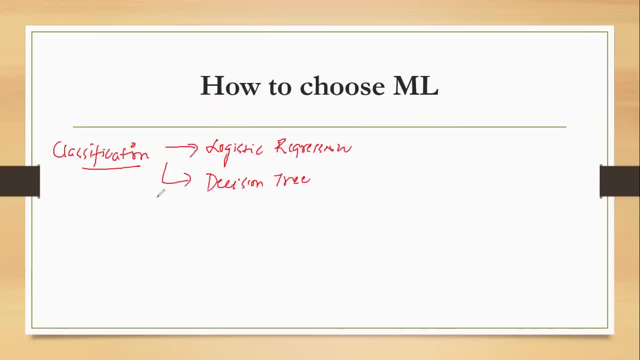 decision trees- okay. the third thing, the third algorithm can be random forest- okay, random forest. the fourth thing can be xgboost, extreme gradient boosting, and these are basically ensemble techniques, guys. that basically means you'll be having multiple base systems. you can have multiple base models in random forest and xgboost. when I say base models, the base, 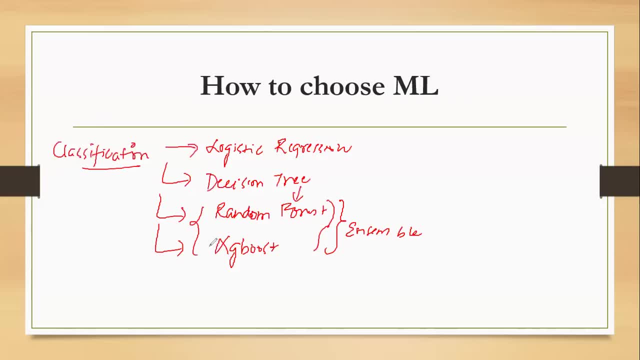 model that is considered within the random forest and xgboost is basically the decision trees, so it will be the combination of many decision trees to solve the problem. you still have other machine learning algorithm, like k nearest neighbor. you have svm and many more. okay, so now you have so many classification algorithms. now suppose you come up with a. 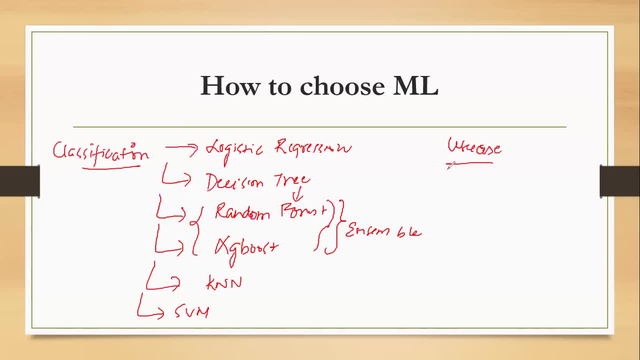 classification use case. now you have a use case. how do you decide? how do you decide, from all this particular algorithm, Which algorithm should we use? right, this is the question that usually comes up, because each and every algorithm has its own advantages and has its own disadvantages. so with what? 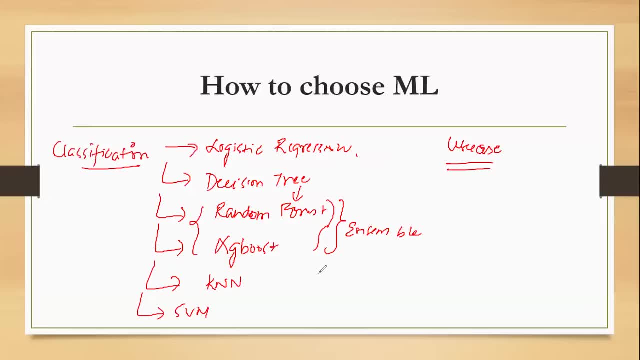 is the best way. should I basically use, or strategies should I use, so that you know I select the best model that will be actually useful for this right now. the one, one, one thing, one. many of them has told that why don't we try all the machine learning algorithm? 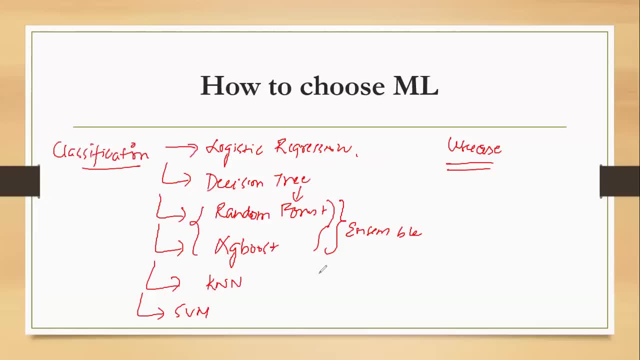 you know, or most of the machine learning algorithm which you consider some of the as the best. Let me tell you, Let me take an example: like decision tree, random forest, xgboost, this three machine learning algorithm guys- I've seen so many developers- this three algorithm are the best algorithm. 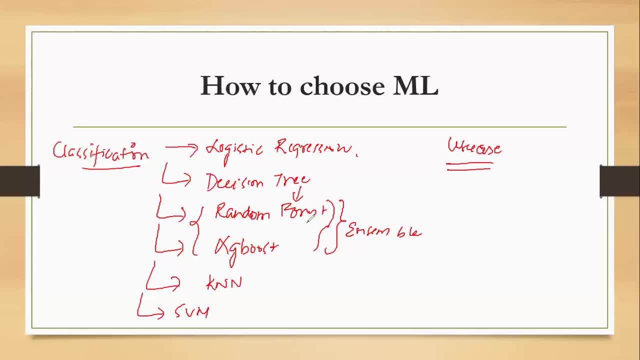 for them. you know all the time they will be saying that if they just see this particular use case, they'll directly say that, okay, just go ahead with random forest, but that is not how we should go ahead. okay, so understand guys, from logistic regression. now, if I, if 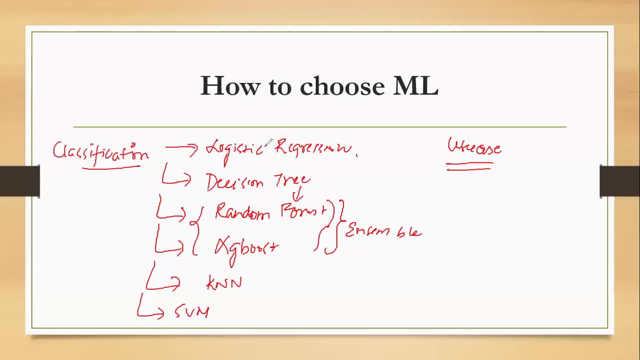 you consider the explanation about logistic regression, if you know about logistic. if you don't know about logistic regression, guys, I suggest you go through my videos in my YouTube playlist. have actually given the exact maths, what is required in logistic regression. but in logistic regression you know the time. 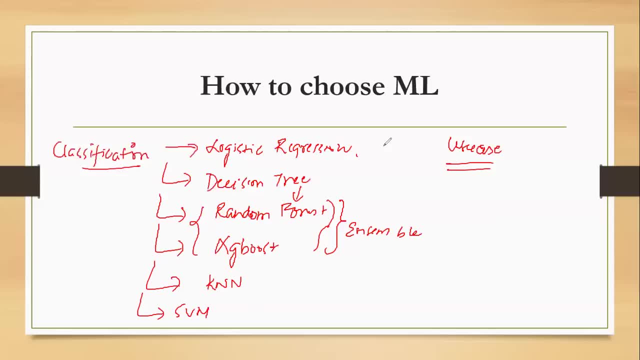 and effort for the model to get trained is very less when compared to decision tree, random forest xgboost. because decision tree you can see that there will be multiple branches that is getting created. it will be like multiple if else loop, if else loop, if else condition. 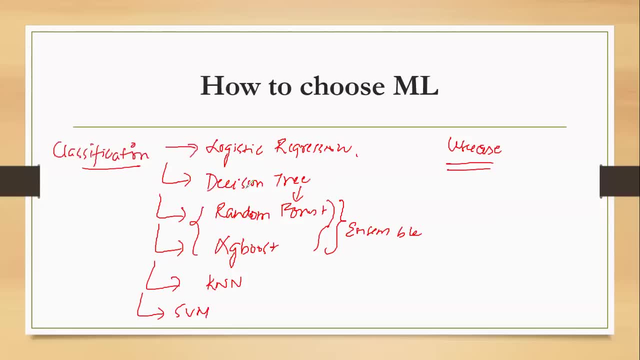 so, based on that, you know, as we go ahead, as we go ahead towards this decision tree, random forest, xgboost- more amount of time usually takes for training the model. now, most of the time in, whenever you are doing a real world scenario, you will be having a data set. you. 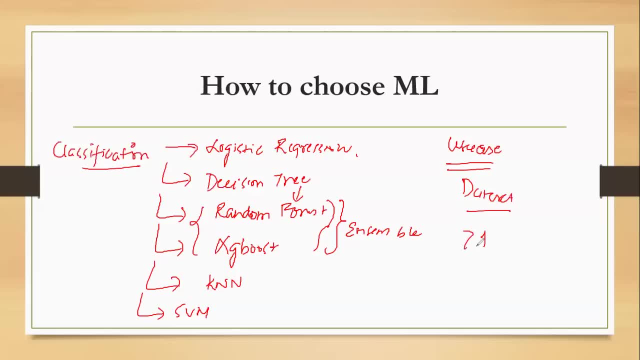 will be having a data set which will be having more than 1 million records. you know, in a training data set you will be having more than 1 million records. and just imagine if you are just trying to apply each and every algorithm and trying to check what is the 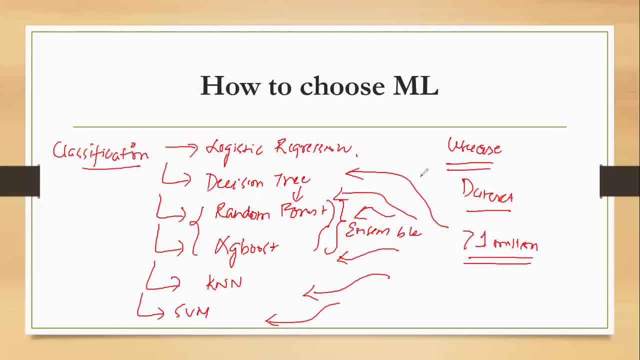 accuracy. it will definitely take much more time right, so it is always better that you apply a technique, a smarter way to decide which algorithm should I use, and one of the technique is basically called as visualization of the data. okay, visualization of the data. now, many of them will be considering: what is this visualization of data? that basically. 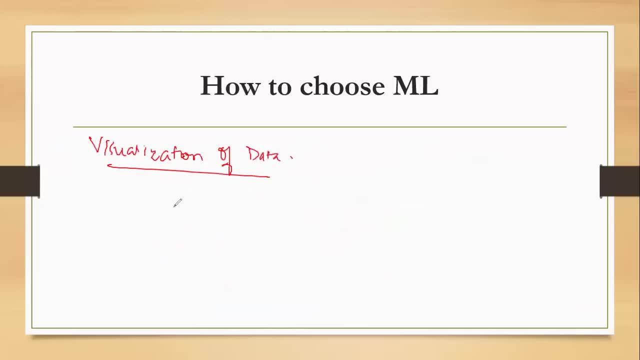 means you are. you are visualizing this particular data through some techniques, and the library that I will basically be using is something called a c1, as soon as I visualize. now, when I say visualization of this data, this the way of visualization, is basically like a kind 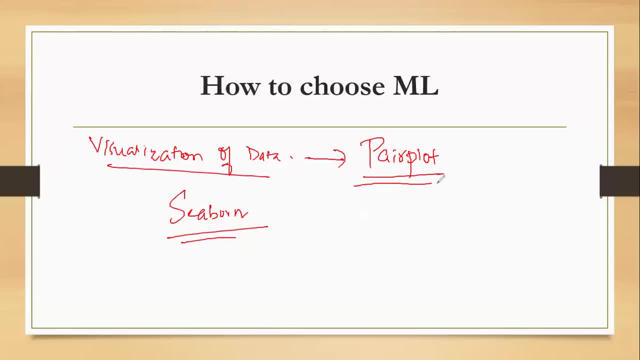 of library by using a pair plot. okay, if some of you don't know what is pair plot, don't worry. in just a minute it will be coming on. I will be showing you the code: how to create this particular pair plot, and for that I will be using a library called a cbon. cbon is one. 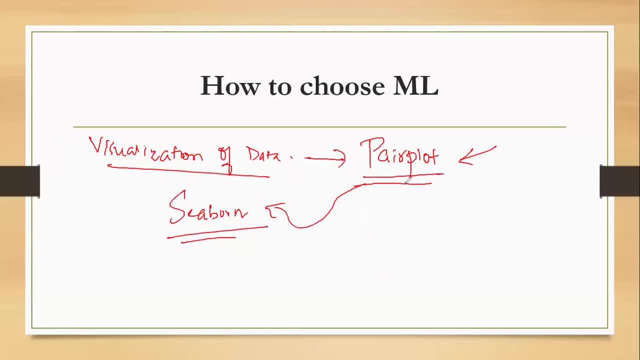 of the best library for visualization of this particular data set that you have and it provides a lot of features like viscous plot, pair plot, you know, univariate plots, bipedal, bivariate plots- all different kinds of plots they have, you know. they help us to calculate the, the 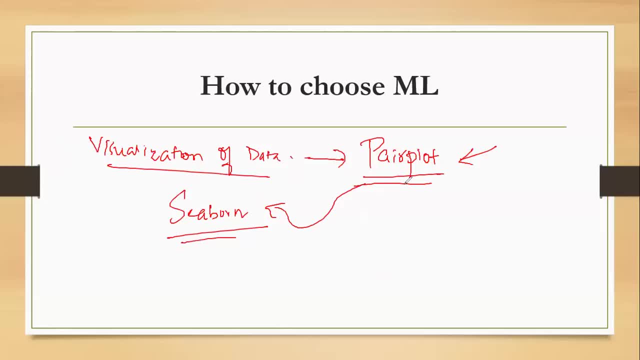 I mean the visualization of the percentiles. also, they provide by using viscous plot, and let us, I'll just show you everything that encoding mechanism. but by applying this particular pair plot, we will be able to understand that which machine learning algorithm I can apply, unless and until you don't know the what that particular machine learning algorithm does. 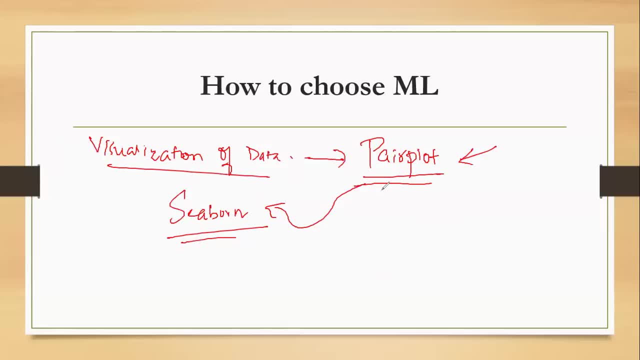 so you should first of all understand, you should basically know, some of their machine learning algorithms with respect to the use cases that you have, and then, by just seeing this pair plot, You will be able to decide that which machine learning algorithm should you apply. now let 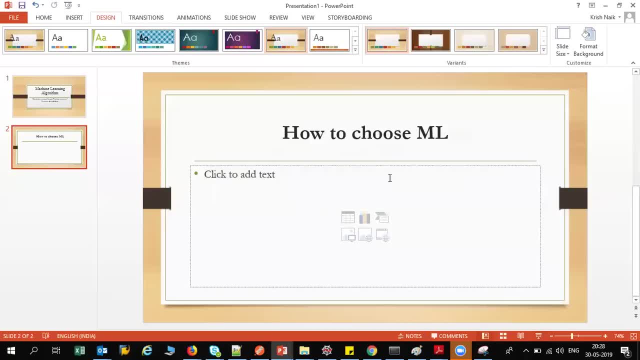 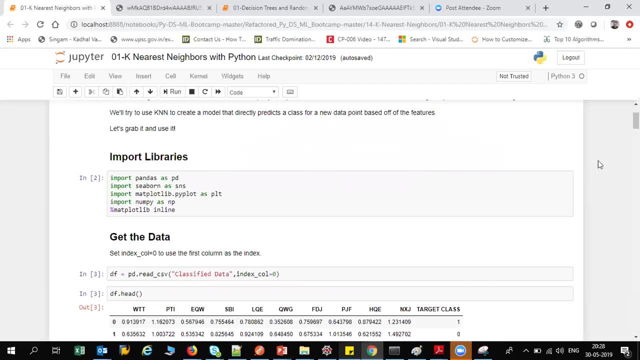 us go ahead and try to see for a particular problem statement. okay, now I'm going to go to the code and I'm going to show to you how a machine learning algorithm can be applied for a particular use case. let us consider one of the example here in this particular 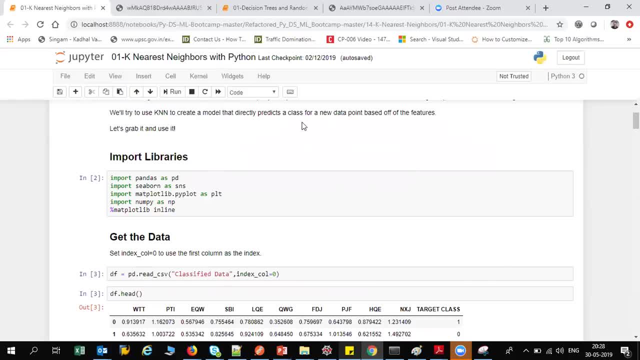 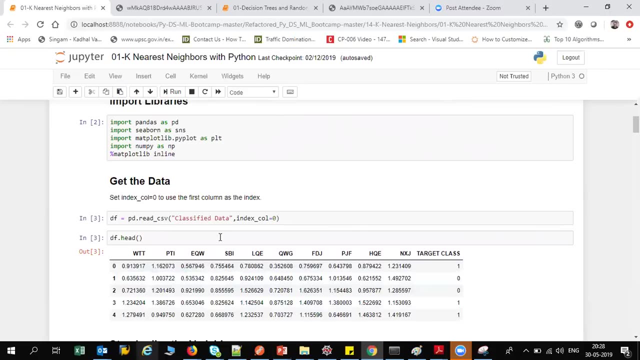 algorithm. I have basically used something called as k nearest neighbor. now, the reason I have used k nearest neighbor. I'll just tell you about that. okay, don't worry about it, but let us just go and read this particular data set. So I have some classified data set of the company, okay, and this data set is just some. 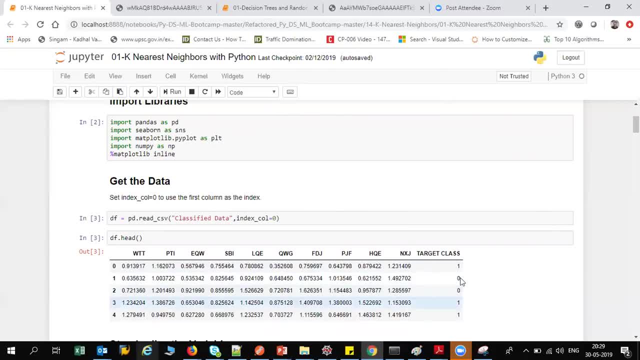 values and integers you can see over here, and there are some target classes you know. now, based on this value, I need to classify this into some target classes. that is what my model should be. so that is all about the use case. Now, since this is a classification problem, because you're dependent, features has two. 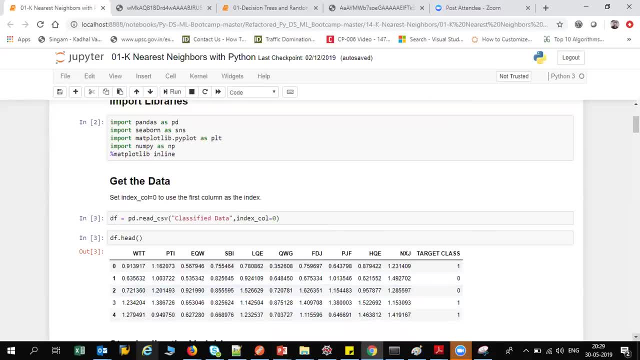 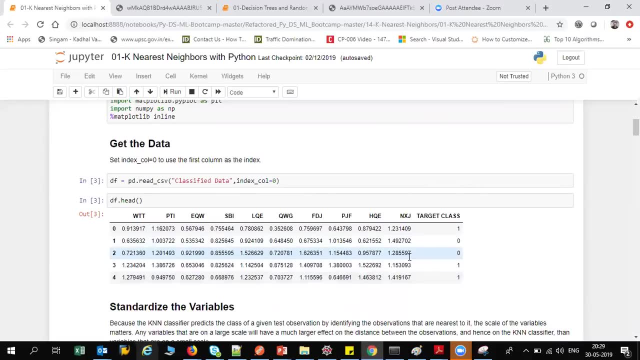 classes, that is, 1 and 0. now how do you decide? how do you decide that? which machine learning algorithm should I apply? apply? I can apply logistic regression. I can apply decision tree. I can apply random forest. I can apply the XGBoost or KNN. right, But now suddenly, why have selected KNN? Let's go ahead. 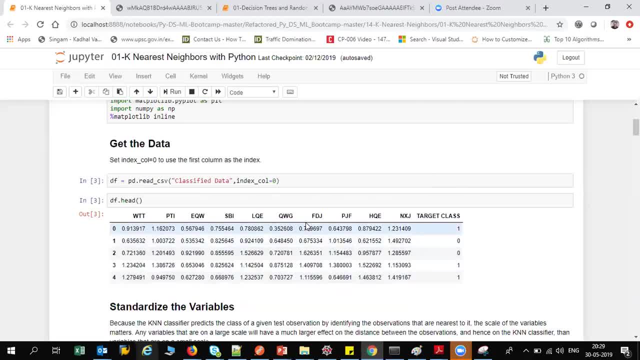 and see. Okay, So first of all, what I'm doing is that I have this particular data set. As usual, I will divide this data set into my independent and dependent feature. You know, my independent features are basically all these columns. Since it is a classified data set, we do not understand. 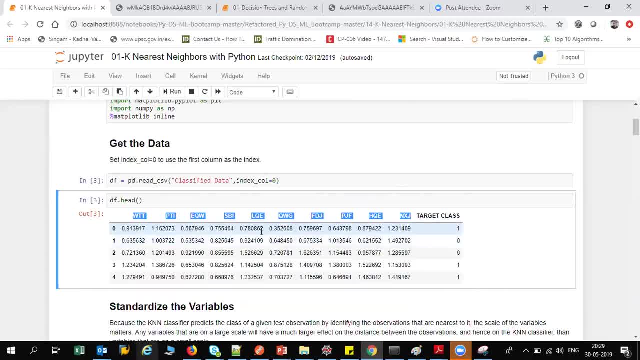 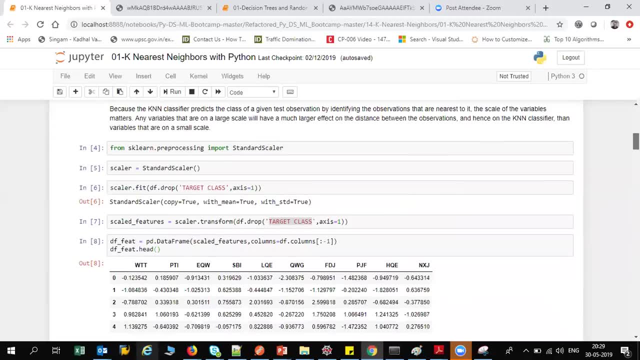 It may be some classified data which gets uh, which the company may be understanding, and they will be this particular target class. Now let us just go and create this pair plot: Okay, So don't worry about the steps. This is basically standardizing. I'm going to scale down. 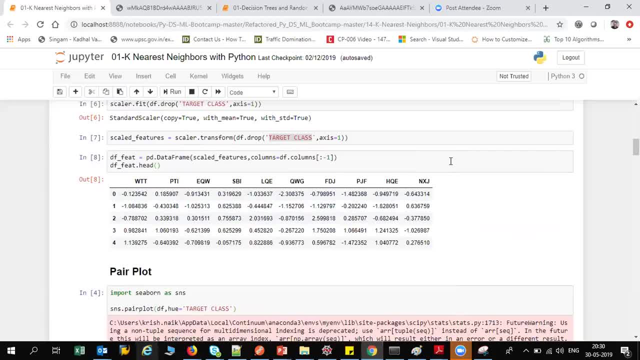 the value with the help of standard, normal distribution. That is what all the steps is done, But anyhow, I'm going to give this code materials. If you want, I'll put up in the GitHub link. it will be put up in the description of this particular video. Now let us go and create the 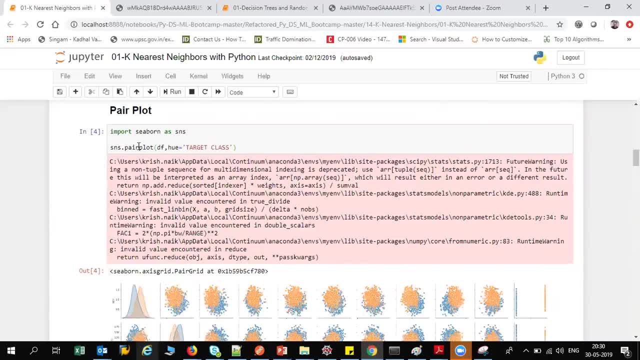 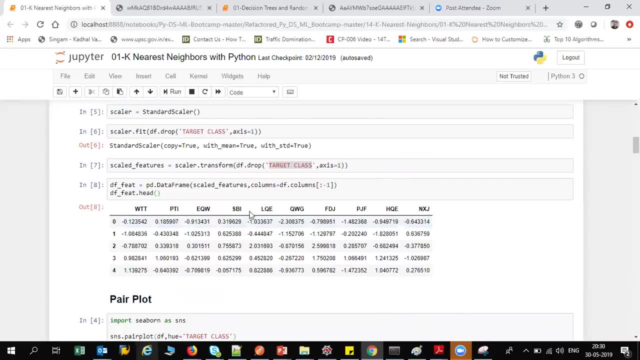 pair plot. Okay Now, pair plot basically means that you understand over here how many features I have. Suppose I have this: WTT features, PTI features, EQ, W features, SBI, LQ, These all features what we 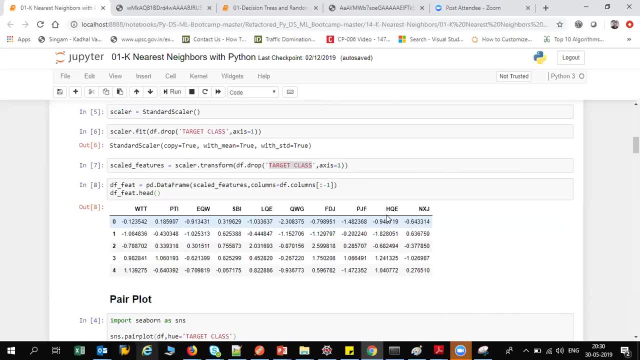 do is that we try to take a bivariate combination. When I say bivariate combination, I will basically be taking WTT and PTI and I'll try to plot both of this particular data in a two dimensional diagram. Okay, Then I will take the combination of all the other data, like 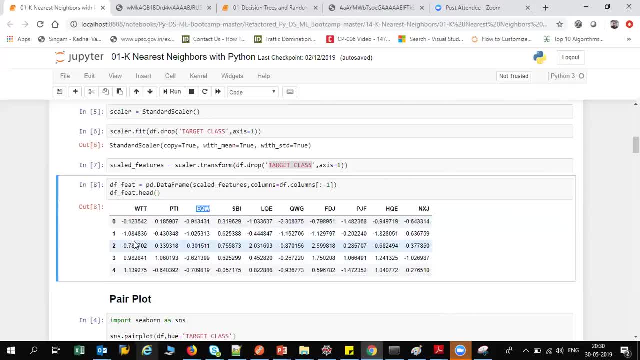 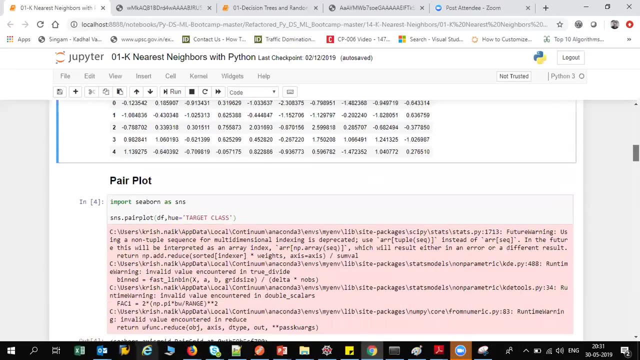 WTT and EQW and I'll try to actually plot it in a two-dimensional graph again. okay, so I will be doing all the permutation and combination of all the features and try to plot a bivariate pair plot. okay, so that will actually help us to see a 2D diagram. in order to do that, we just have 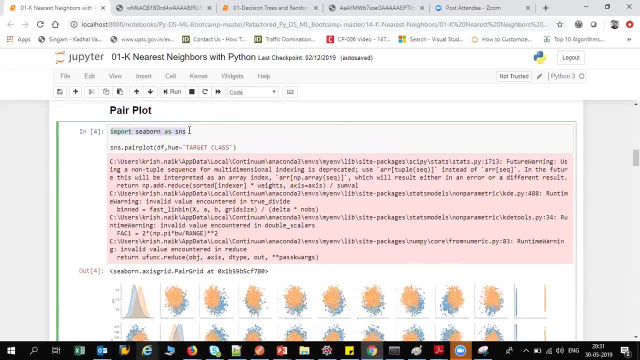 to import CBON now. CBON is a very popular visualization library, so make sure you have some knowledge about CBON, you know, and in this CBON there is a functionality which is called as pair plot. now, inside this pair plot, all I have to do is that I have to give my data set DF. 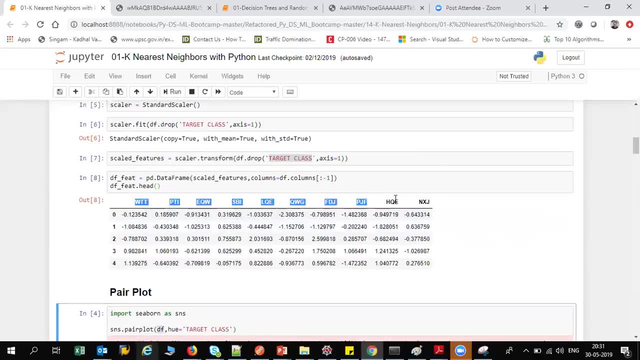 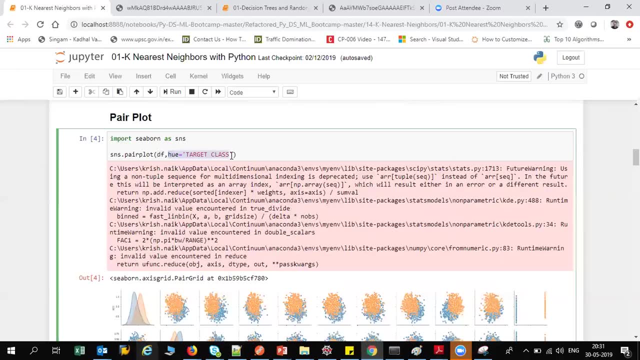 now, this particular data set is basically my complete data set that I have over here. okay, now, as soon as I give this particular data set, then this we parameter says that, since this is a classification problem, now when I'm seeing the pair plot, I should be able to see which all. 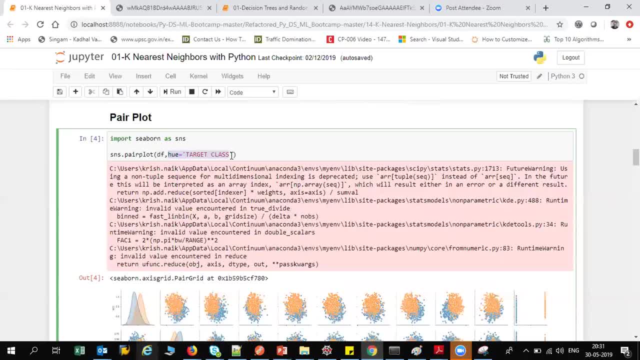 are one and which all are zero. okay, which all are one and which all are zero. so for that I have to give my data set DF. now this particular data set is basically my complete that case. what I'm doing is that I am providing that it should be classified based on the target. 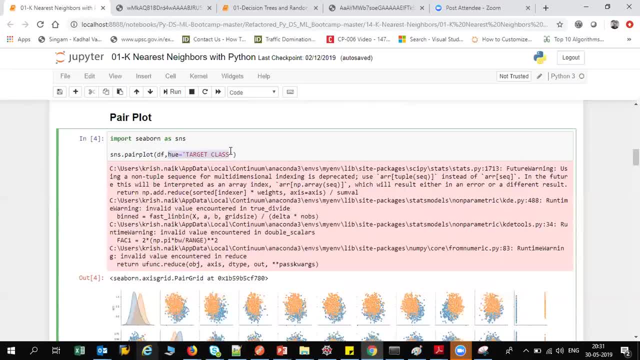 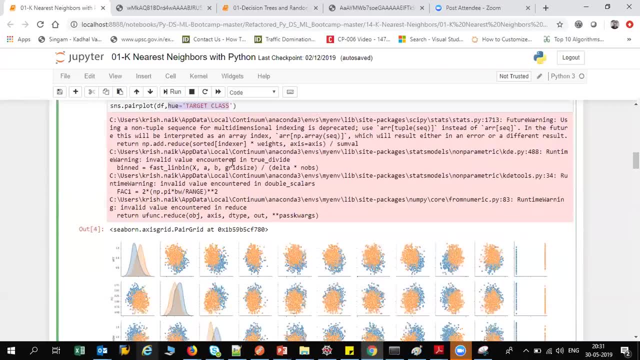 class. so I have actually given this we parameter. now see this guy. as soon as I put this, the magic will be that I will be getting this kind of graph now. don't worry about this. warnings guys. this is because of the current version 3. I'm working in 3.6, but if you execute this in 3.7, it will work. 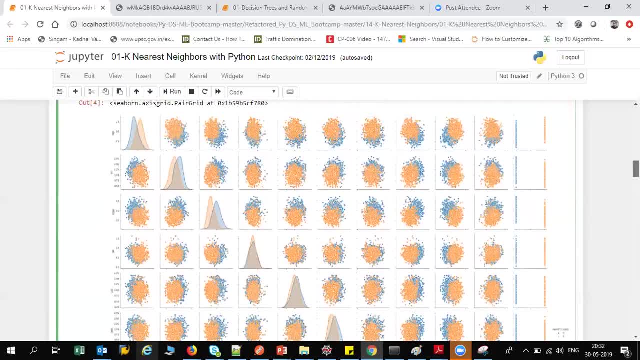 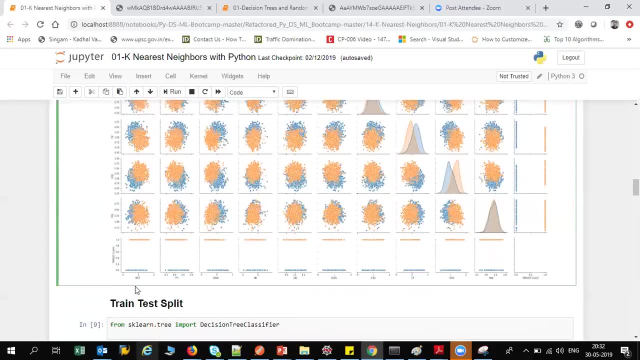 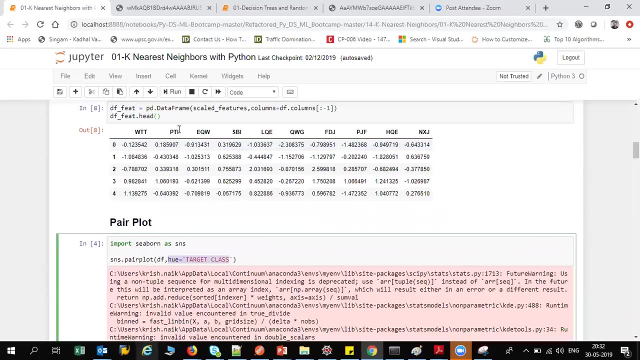 perfectly fine. okay, now, as I go down, you can see that I have this particular graph. now, one thing you have to note about this graph, guys, is that this graphs in the x-axis, in the x-axis. always. remember that we will be getting all these features like WTT, PTI, EQW, SBI, LQE, QWG, FDJ, PGF. 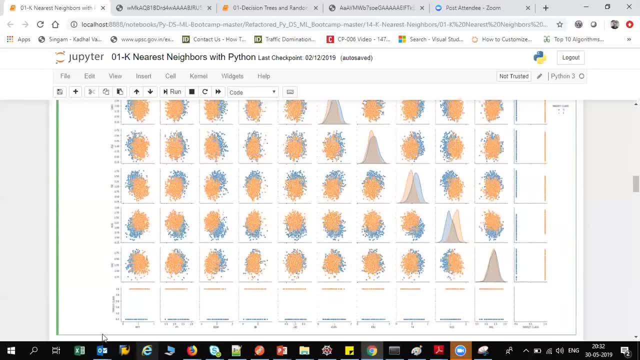 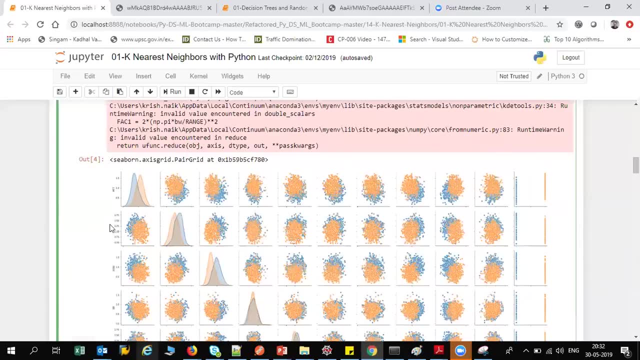 HQE and Excel. so all this will be present in x-axis, right like that. similarly, all this features will also be present in the y-axis, like it will start with WTT, PTQ, EQW. it is not visible at all, so it will be present in the y-axis. so it will be present in the y-axis, so it will be. 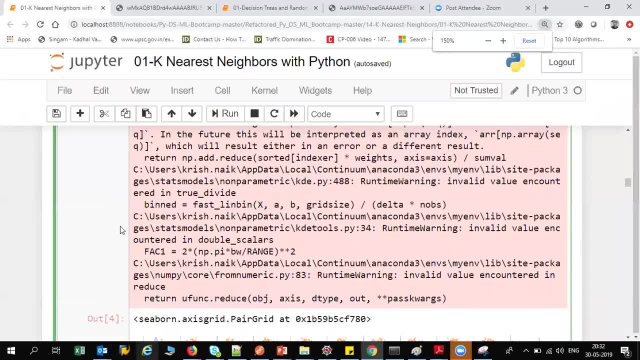 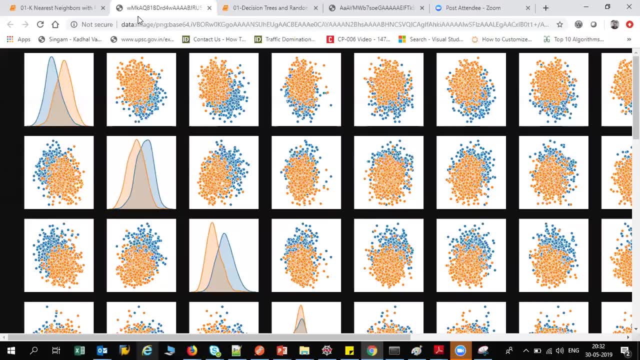 and I think I'll also not be able to zoom completely. let me try if I am able to zoom. so the image is not getting zoom. what I can do is that I can open it in a new window if you want. so the images will look something like that, but still I'm not getting what is there in the x-axis. 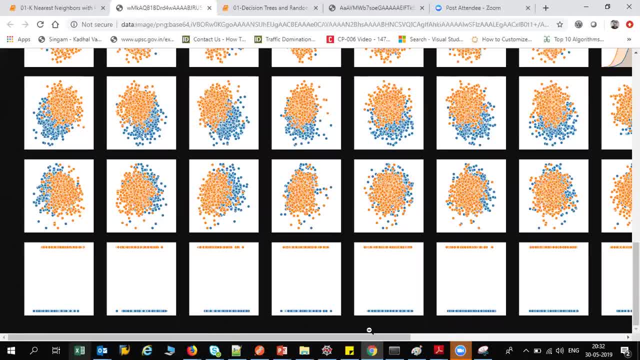 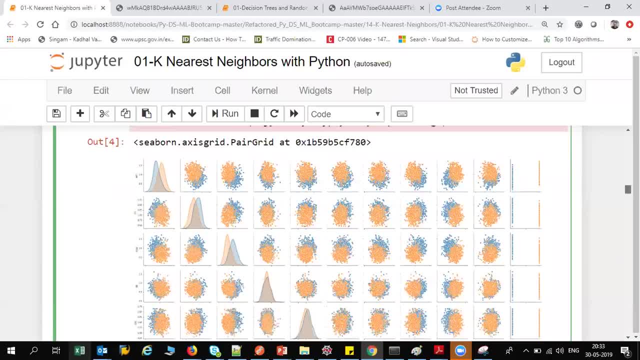 and y-axis, but just understand, x-axis will have all the features that are present in the column. similarly, y-axis will have all the features that are present in the column. now, when I see this kind of graph- okay, this kind of graph- you see that in the diagonal, elements are present in the 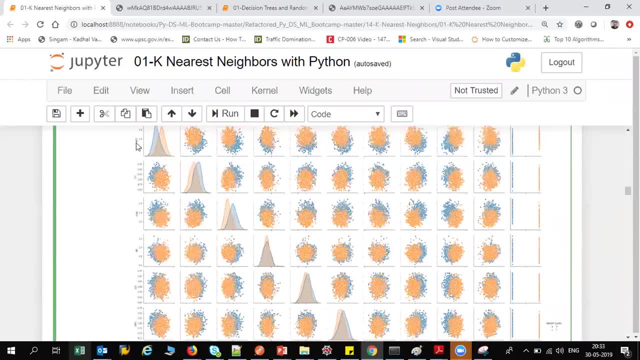 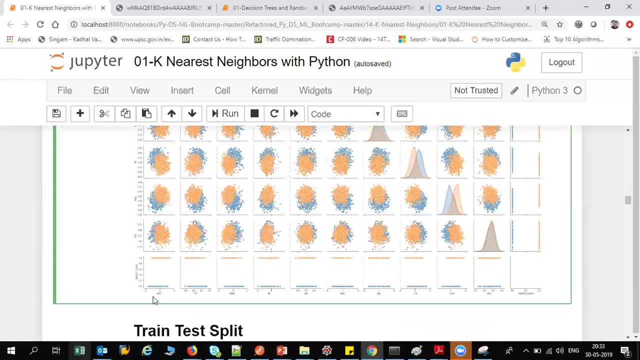 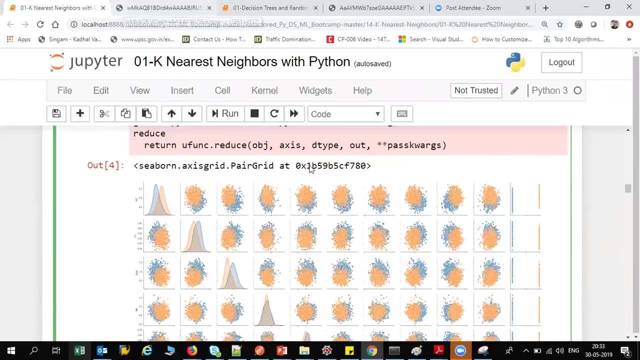 last four elements, you will be getting this kind of PDF functions. okay, this PDF function is basically because of WTT versus WTT in the x-axis- WTT in the x-axis- okay, so don't worry about it just now. what it has done is that it has done all the permutation and combination and it has created 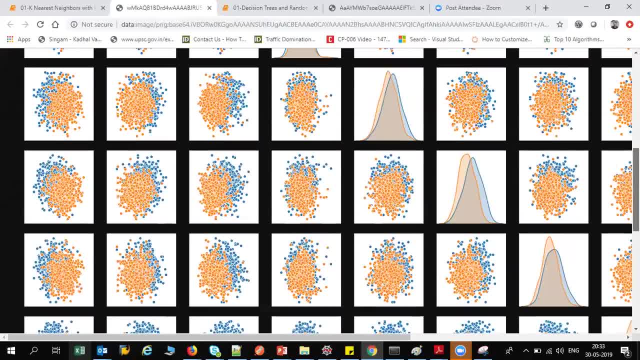 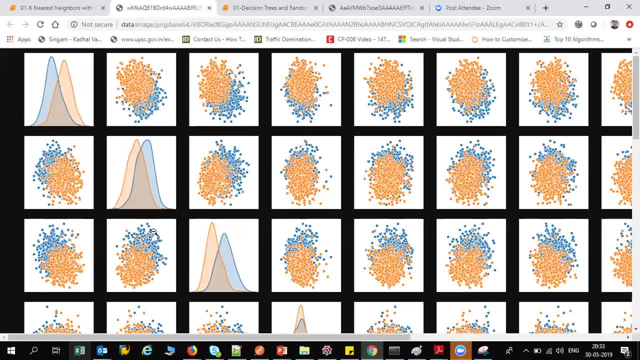 this kind of figure, this kind of figure now you can do. you observe something very familiar in this particular data. now just try to solve this particular information. okay, let us just take two features and try to see that, if you have a particular data, okay, you can solve this particular. 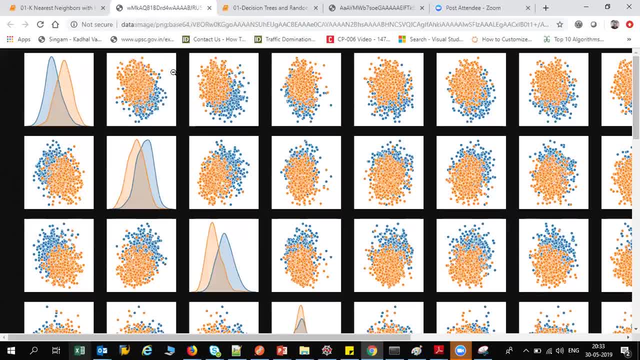 how can i solve this classification problem? okay, this is the most important thing, guys: how can i solve this particular classification problem? now, you see that there is a lot of overlapping, okay, between the points that are classified as target one and zero. so, first of all, let us go. 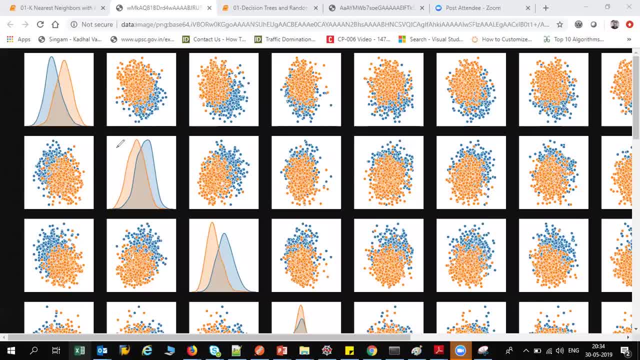 with the first algorithm that you basically know is basically called as logistic regression. can i solve this by using logistic regression? now understand the concept in logistic regression, guys. in logistic regression, what the algorithm does is that it tries to create a straight line to do the division of the data, to do the division of the data. now just imagine if i just create a. 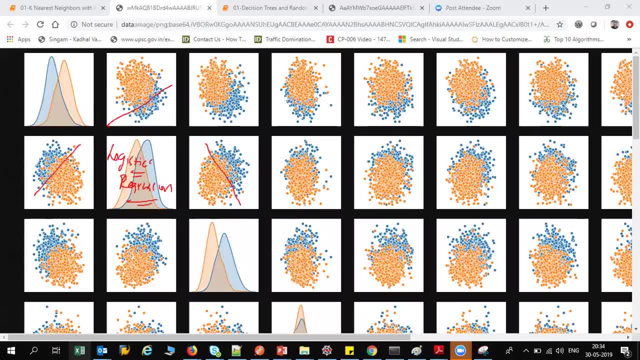 straight line and i'm trying to classify the points. how much is the error that we may get? what will be the accuracy level? just by visualization you can see it, guys. see, there is a huge amount of overlapping here, here, here, similarly, here also, we have huge overlap. 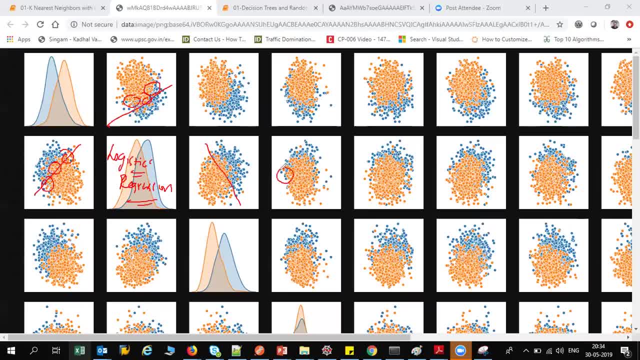 overlapping right. it is very difficult for us. if you just apply logistic regression, we may not be sure that it will give us a very good accuracy, because there are a lot of overlapping guys. you can't just draw a straight line because there are a lot of points over here and we don't 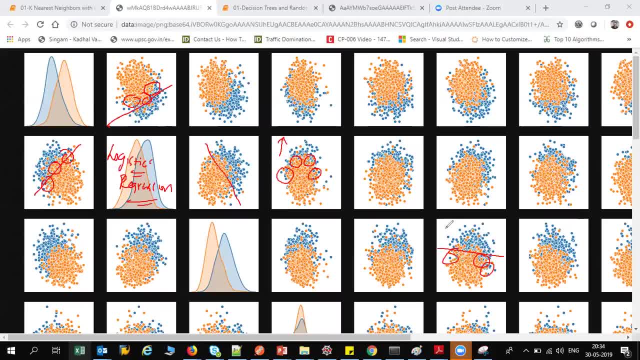 know like how many points right. so there are a lot of overlapping. so it is now definitely true that you cannot apply logistic regression, because the error rate will basically be high. okay, when you do a train test split and then when you try to find out what is the test value for that which? 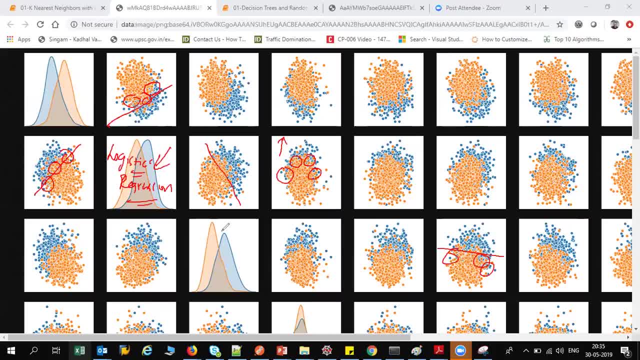 point it is getting classified, definitely the accuracy will be very, very less because the data is not distributed properly. it is having a lot of overlapping. now suppose, if i take one more example where my data was distributed somewhere like this: suppose this is one mic, one of my class, okay, this is one of my class and my other class was somewhere like this: 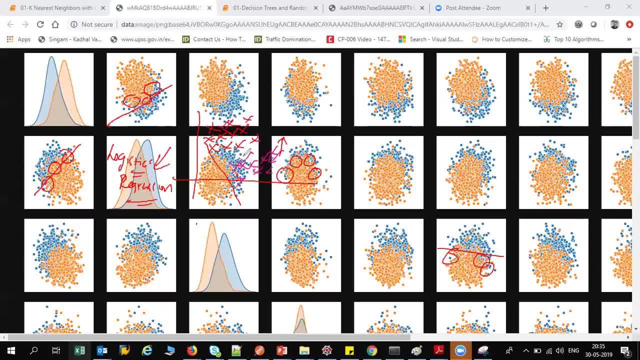 right, suppose my other class was somewhere like this. okay, and then when i take one more example where my data was distributed somewhere like this, then i can draw a straight line in there into this, because this of this, these points that i have, is not overlap, right? these are clearly indicated that they are present in a separate. 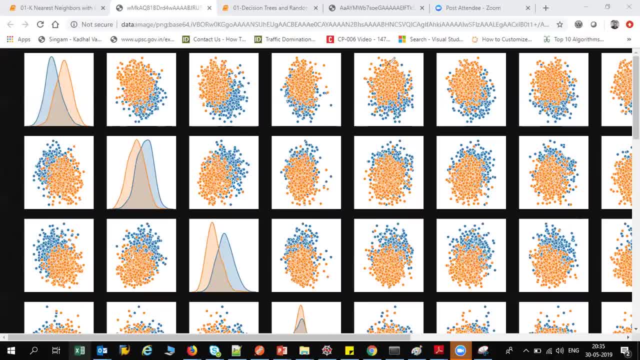 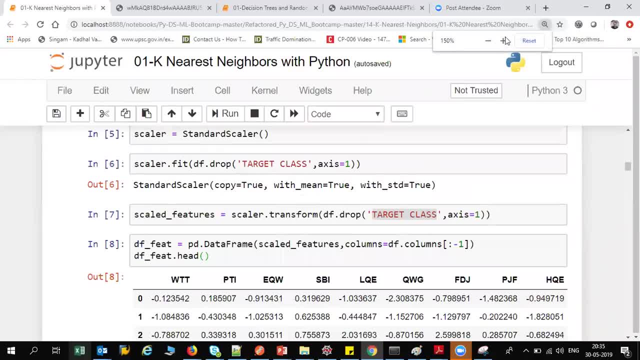 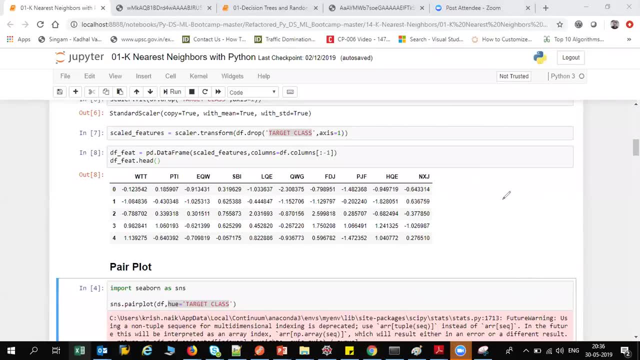 windows. now let me just show you once more in the diagram over here. okay, now suppose just imagine that i have a data set. i have a data set. suppose it is in this way. just let me just show you once. suppose i have this particular data set. okay, and one of my 2d diagram is somewhere like: 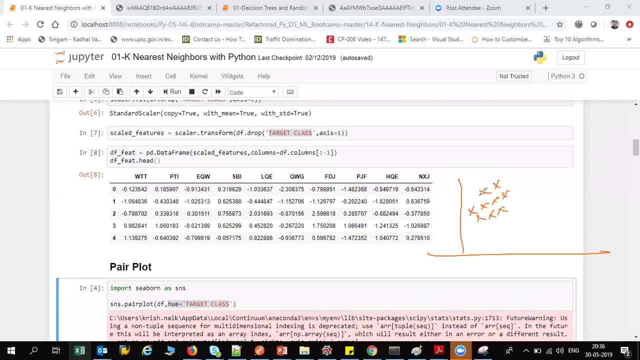 this. i have some points over here, you know, and some points over here right, if i have this kind of points like this, now you can see that there is less over overlapping, right, so definitely you can apply logistic regression because you know logistic regression basically applies a straight. 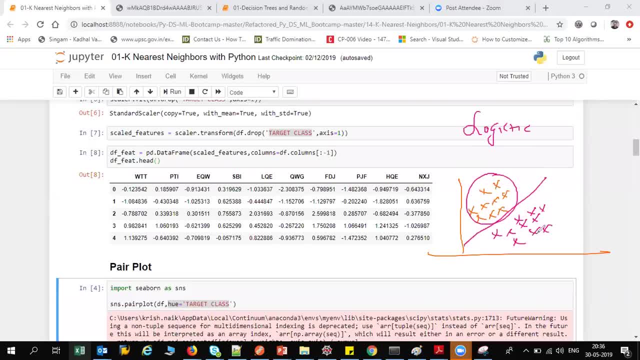 line. it creates a best fit line which will be able to divide this two parts, the points very clearly and the accuracy error error accuracy will be very, very high in this case because there is no overlapping for this. i think you should not go because you know that. 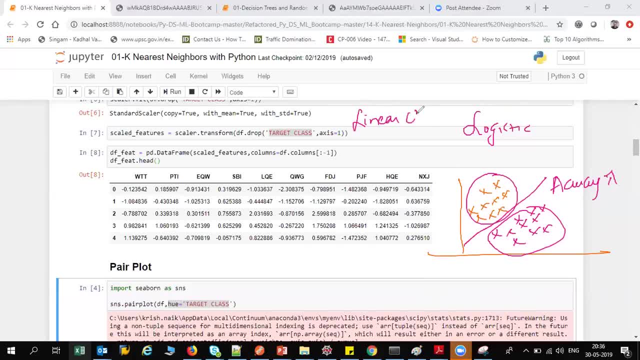 logistic regression is used for solving linear classification problem statement, linear classification problem statement. but when you consider about decision tree right, or when you consider about random forest in classifiers, or when you talk about knn, these all are able to solve non-linear classification. non-linear classification basically means that 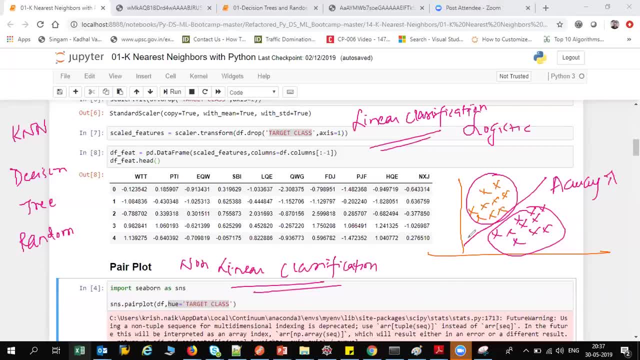 if your data has overlapping. even though your data has overlapping, it will find out a way to classify that points through some way. okay, so this is this is how these things work, you know. so, basically, knn decision tree, random forest- is basically used for non-linear classification. 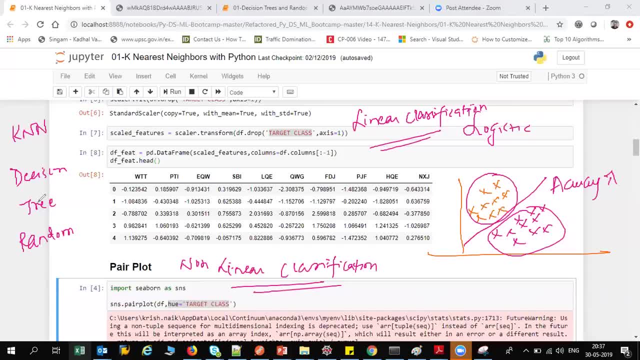 whereas logistic regression is used for linearly classification. that basically means that logistic regression will try to create a straight line for dividing these particular points and this will just act like a best fit line which will be clearly able to, you know, classify this particular points, whereas in case of knn- decision tree, random forest- there will be different, different. 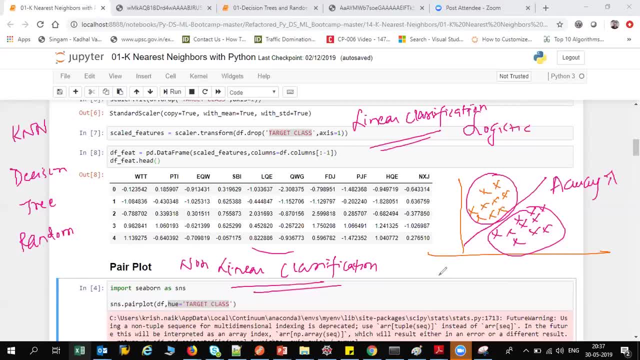 kind of non-linear shape or non-linear way. non-linear way basically means that my curve may move something like this to divide the particular data set. it may not be in the straight line now from this particular diagram. you see that from the graph that i saw over here, or the 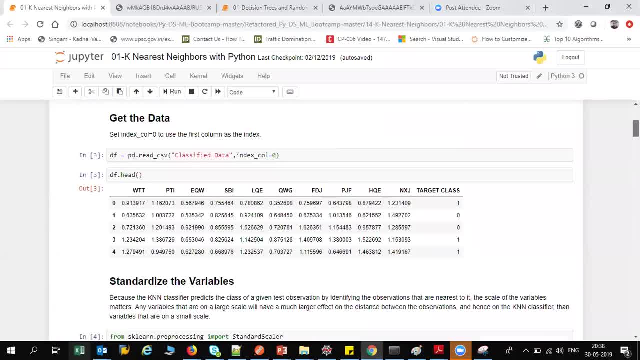 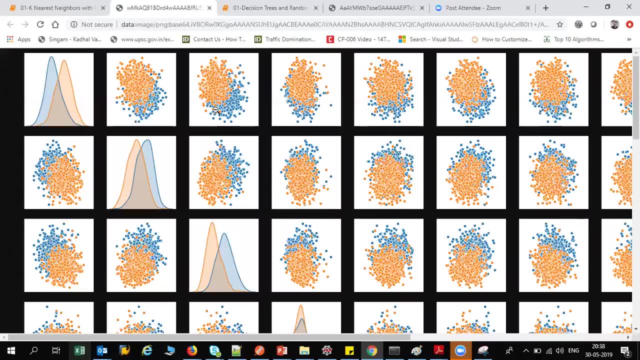 or the image from the pair plot. it is definitely certain that you will never be able to apply a logistic regression because the data points are too much, you know, overlapped within each other. So definitely. So one thing is that I have skipped out logistic regression. 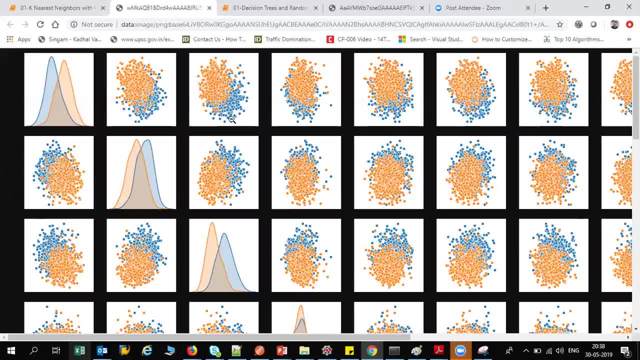 Now the next thing is that: can I apply decision tree? Can I apply decision tree? That is the next question. Now, when you talk about decision tree, random forest and XGBoost guys, you can definitely use this, but always remember decision tree. 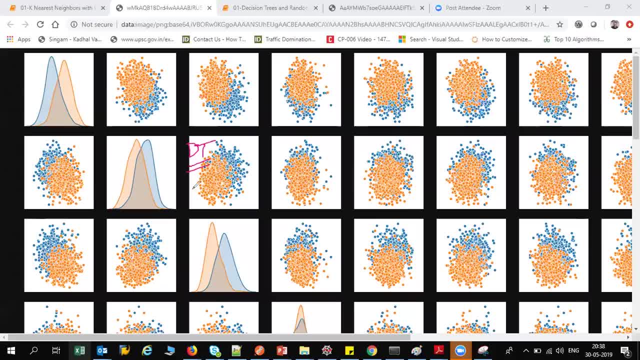 random forest and XGBoost also requires much time, you know to train their model. It requires much time because decision tree is nothing but multiple nested FL slope right. Definitely you can apply decision tree, but always that there's a disadvantage in decision tree. 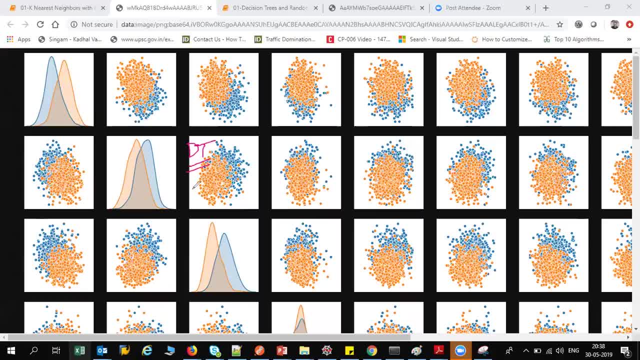 What the structure may go like. the depth of decision tree may go up or you can also apply a different kind of techniques where you can reduce that depth. find out the actual depth by using grid or CV, randomized or CV, So one. 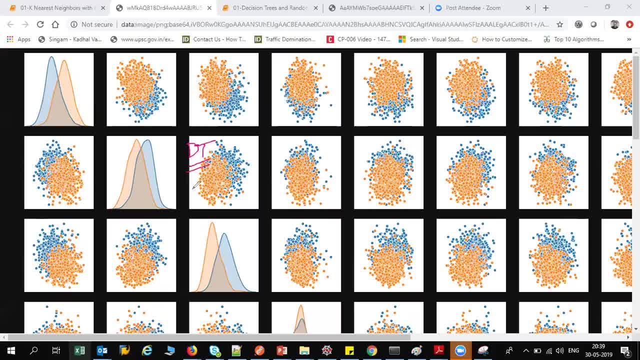 one scenario is that definitely to skip logistic regression because this is a lot of overlap. The second thing is that you can start with decision tree, you know, or if they are much overlapping in your data set, like your data set is completely overlapped. 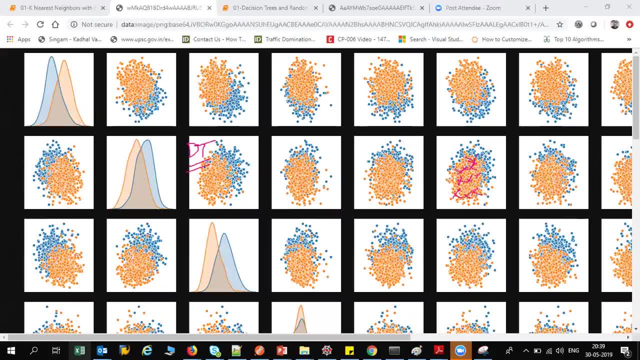 It is present here and there in don't know what kind of thing can you you can apply If there is a lot of overlapping. you should definitely prefer using KNN. Now again, guys, why I'm saying KNN? because KNN uses a concept of Euclidean. 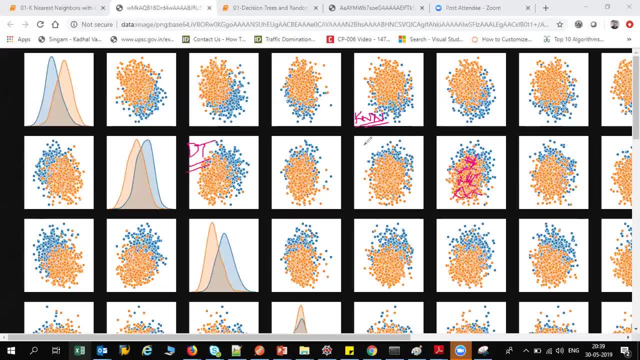 right. It uses Euclidean distance to find out the similarity of the points where it belongs to right And you know, based on the neighbors that it has, it'll try to find out the similarity based on the Euclidean distance. So if you have a lot of overlapping of a data points, 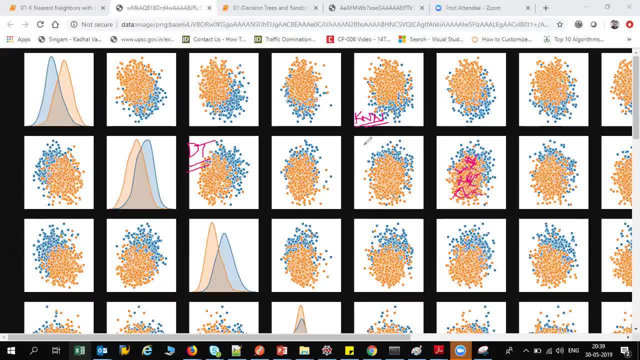 there's definitely going to apply KNN and you don't have to worry about that. No, but if, if still, you feel that KNN is not performing well, then you prefer going with decision tree, random forest: next you boost: no. 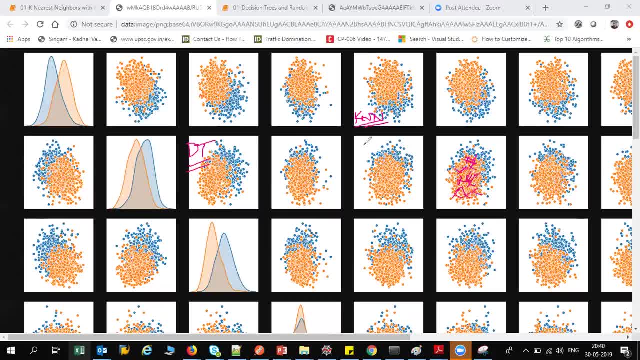 but the most costliest, you know, will be random forest or XGBoost. you know, because the depth of the T tree, suppose. if you take that in decision, in random forest you want to create a hundred trees. So based on this particular data, 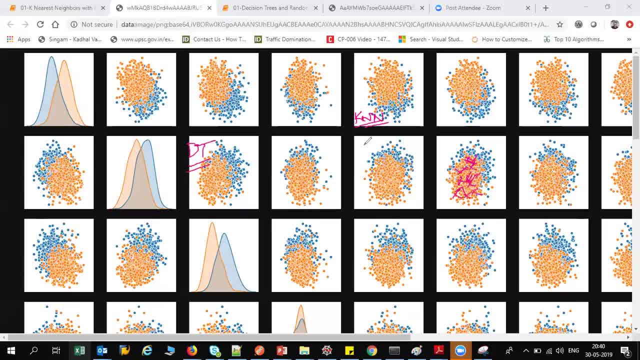 you'll be creating so many trees. but I've seen guys they don't even try with KNN. They don't see that. See, the one point is that if the data is not overlapped too much, you can definitely go with decision tree and random forest. 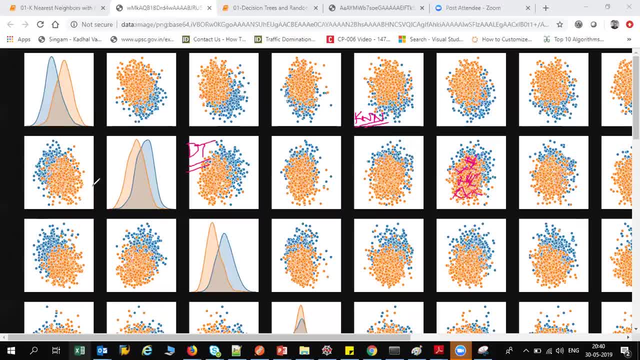 But if your data is completely overlapped, you know now, here also, you see that the data is overlapped. overlapped because you can see that most of the data is present below This, this orange data also. Okay, So that is the reason why I have applied KNN in this particular problem. 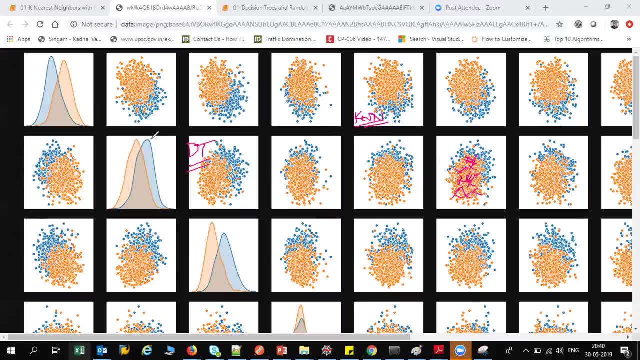 statement You go and try and apply with decision tree and random forest also. I also did that, but the accuracy that I found out when K nearest neighbor was more. So this is the best thing that you understand from this. Okay, So this is how you have to find out. 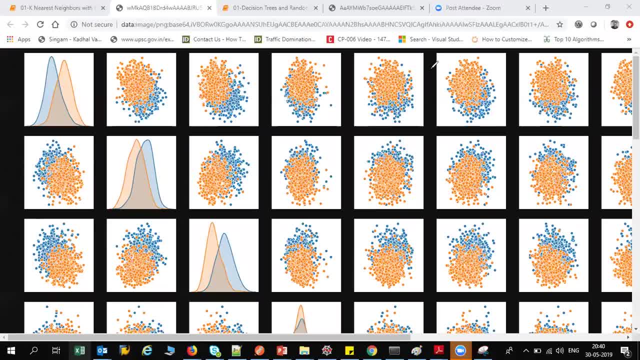 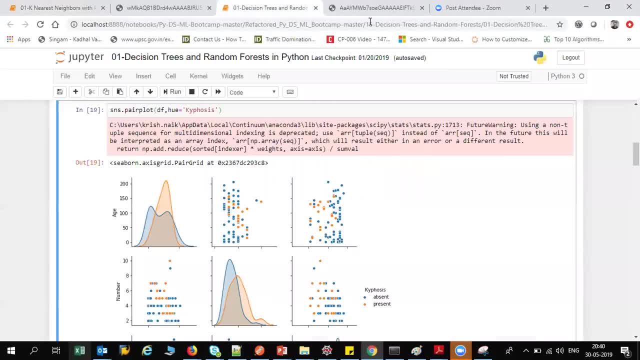 You have to find out a way. Now let me just show you one more example, a simple example a, wherein we will try to see for a decision tree or a random forest. Now, this is one of the graphs that I get from this particular data set, and let me just zoom out this particular. 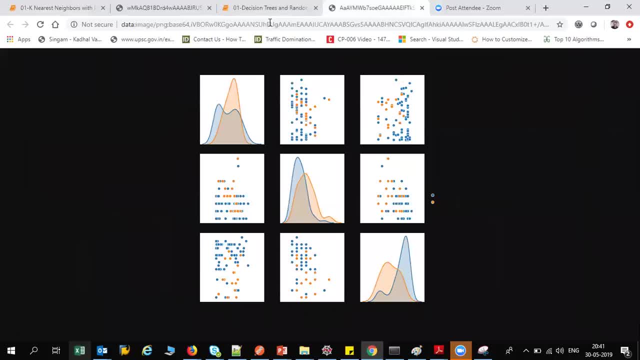 data like this. Now, just tell me what kind of algorithm you want to apply in this. Now, definitely you cannot apply a logistic regression, because you cannot create a straight line, Okay To divide this particular data points. Definitely you can't do that. 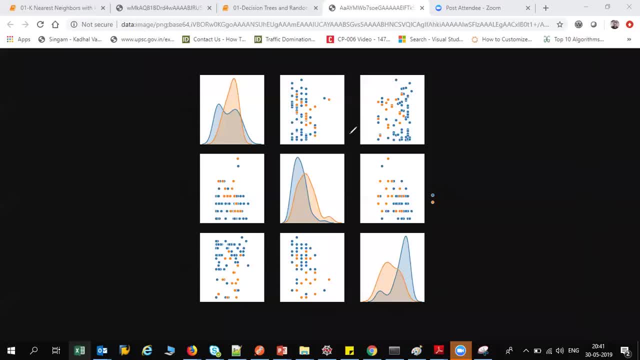 Now the other thing is that you can definitely apply decision tree, random forest, exe, boost or KNN- right, Because all this particular scenario will work for this algorithm, because decision tree is all about making different, different groups, like multiple, if else. 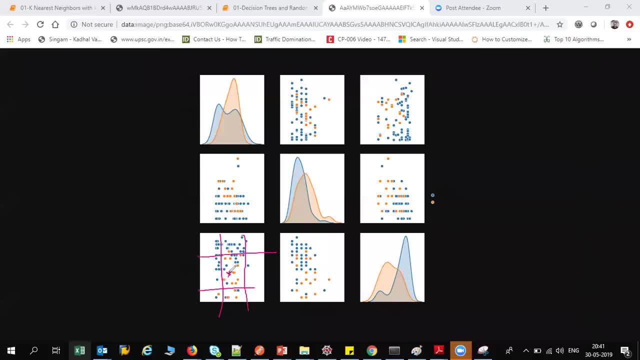 loop something like this. I suppose a new data point comes to this. then you will be able to identify that which classified point it belongs to right. So all of this particular scenario works well, but you need to find out this pair plot.